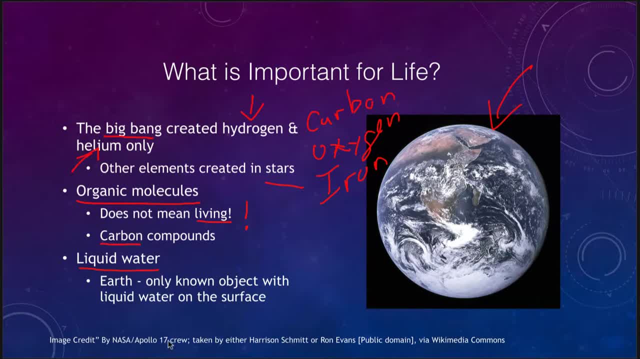 And the other thing we want to look at is liquid water. Is liquid water very important? And this is the only known object with liquid water on the surface, just this one, And we picture it here. that is our Earth. We know that Mars maybe had liquid water in the past or did have liquid water in the 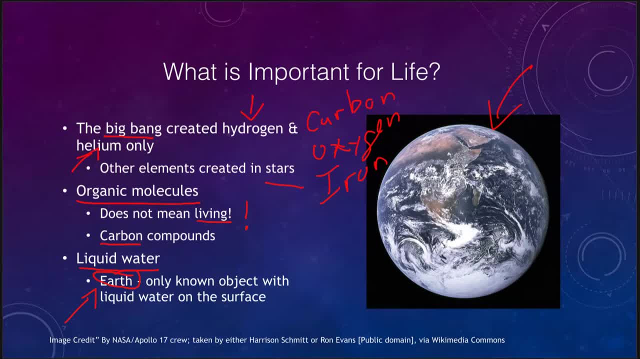 past, And there may be other planets outside our solar system that have water, But this is the only one that is known to have liquid water on its surface currently. So let's look a little bit here. What do we mean? One of the things we sometimes talk. 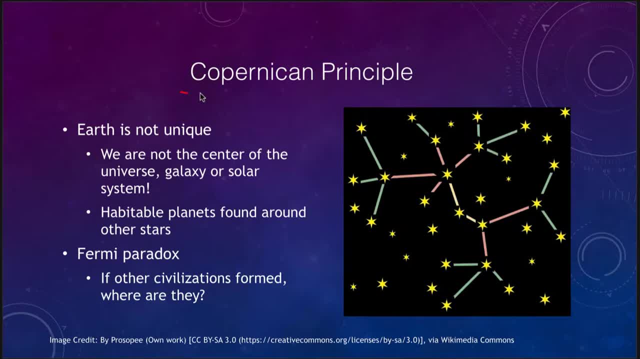 about is what we call the Copernican principle, And what that means is that the Earth is not unique. So we're not the center of the solar system, We're not the center of the galaxy, We're not the center of the universe, We're not the center of anything. So when we talk about 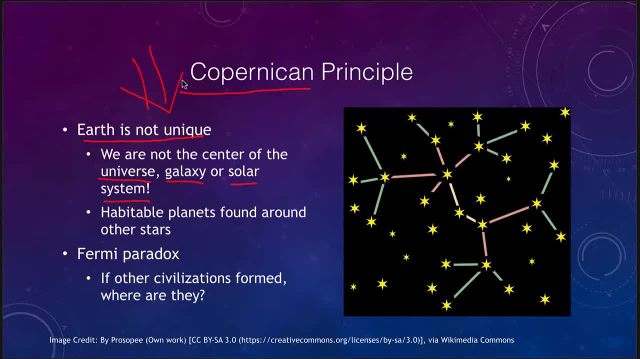 the Copernican principle. we're really saying that the Earth is not something unique, That there are lots of habitable planets out there and there could be more Earth-like planets out there in the universe. In fact, we've detected a number of Earth-type planets. We just don't know whether life has. 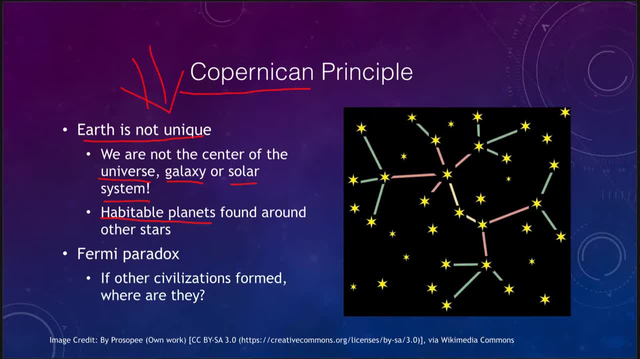 evolved elsewhere, And one of this leads rise to a paradox that we call the Fermi Paradox, which was proposed by Enrico Fermi, And he suggested that you know, if other civilizations formed, why haven't we found them yet? Why are they not here visiting us? if other civilizations formed? Because 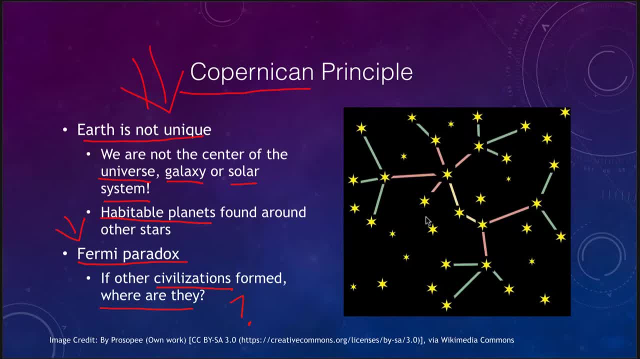 what would happen very quickly, kind of shown in the map here, is that when a civilization formed on a star and developed space travel, it should be able to colonize other planets very quickly, And then those would colonize other planets around other stars And over. 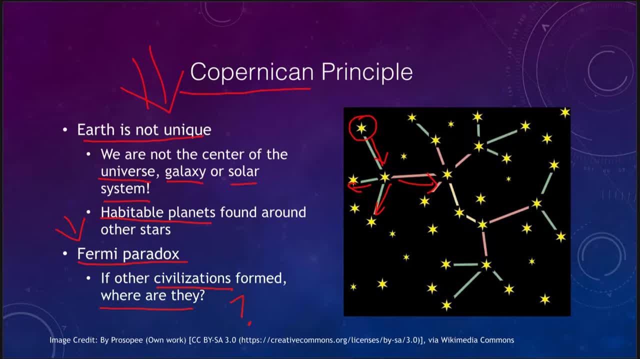 relatively short times, galactically speaking, meaning many millions or even hundreds of millions of years, that civilization would expand out and cover the galaxies. So in reality there should be civilizations all over the place. So what we may mean is that maybe this travel is a lot harder than we think it might be. 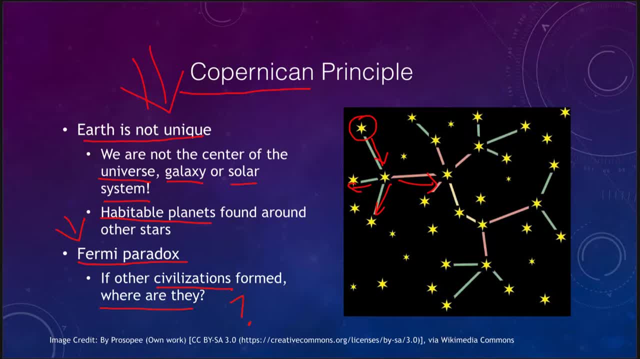 or that science fiction would lead us to believe That. you know, maybe there are easier ways to travel, Maybe there are not, Maybe it is very difficult to travel between the stars, But even things that would be technologically capable now are not something or would still. 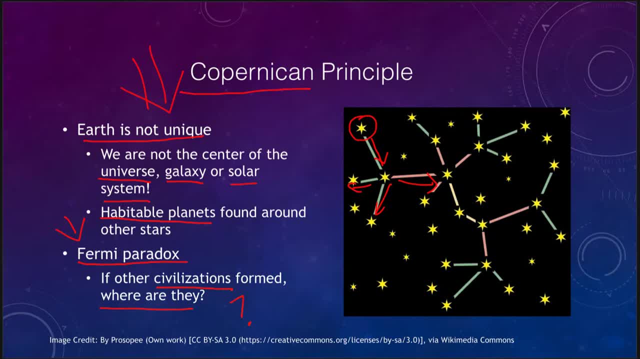 be able to explore the stars, at least the nearby stars, Over things like millions of years. you would be able to travel that kind of distance there. So it is a big what we call a paradox as to why these other civilizations have not. 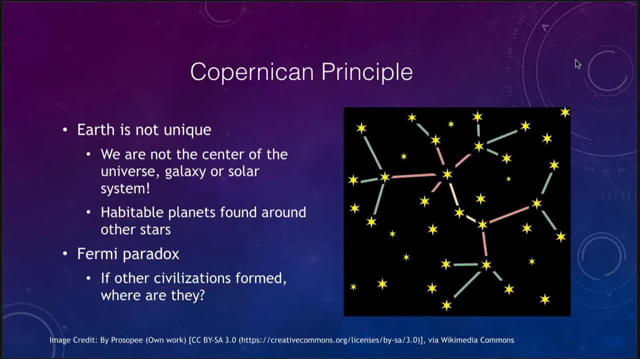 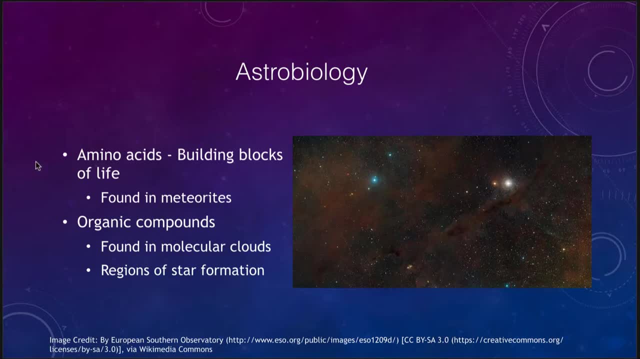 yet been detected. So let's go and look at what we mean by astrobiology or the biology of astronomy, And one of the things that we look at, one of the things we talk about, are amino acids. Amino acids are the building blocks of the universe. They are the building blocks of the universe. They 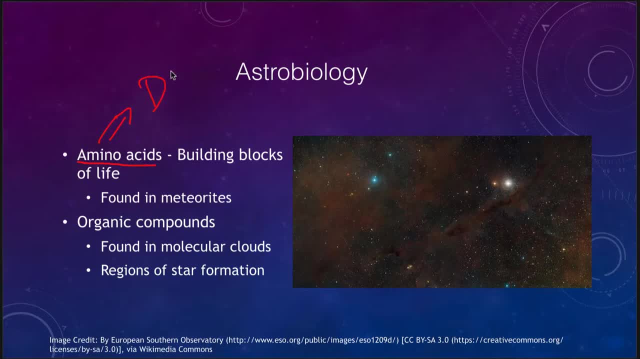 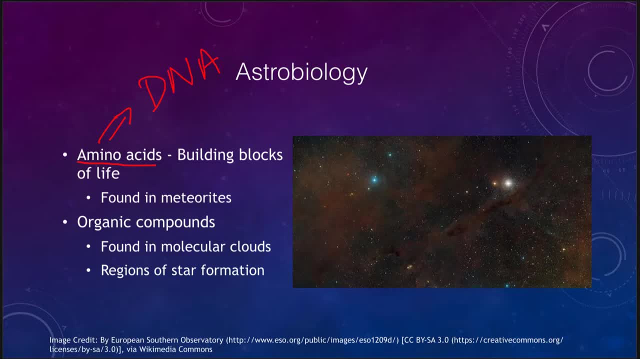 creature. So the amino acids are the building blocks of that and they are very common. They are found in meteorites, and other organic compounds are found in things like molecular clouds, dark regions. here that we see, We can actually detect the emissions of organic. 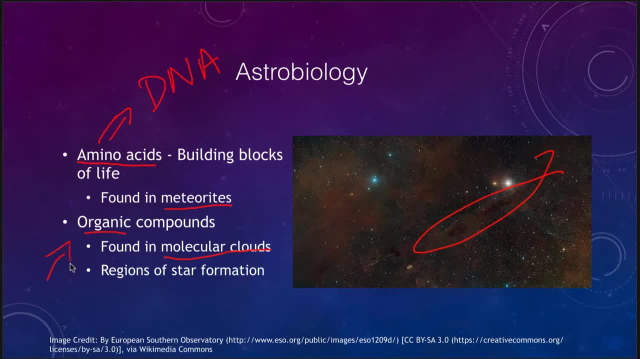 compounds. So we know that organic compounds form very easily in regions of star formation, leaving the possibility that they could become parts of newly forming planets. But how about looking within a planet? How easy is it to form these amino acids which could then possibly lead? 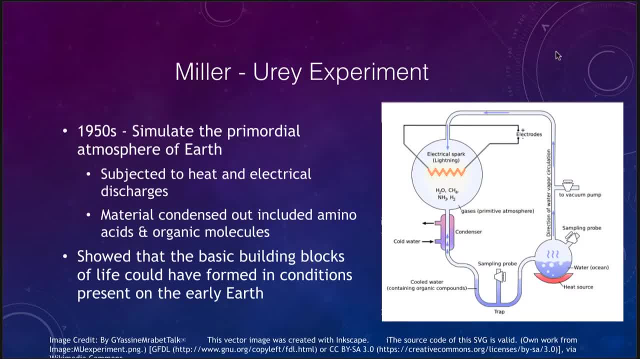 you to DNA, And one thing we look at that is an experiment that was done in the 1950s was the Miller-Urey experiment, And what that did was to simulate the primordial atmosphere of the Earth, So not the atmosphere that it's made up of today- nitrogen and oxygen primarily, but 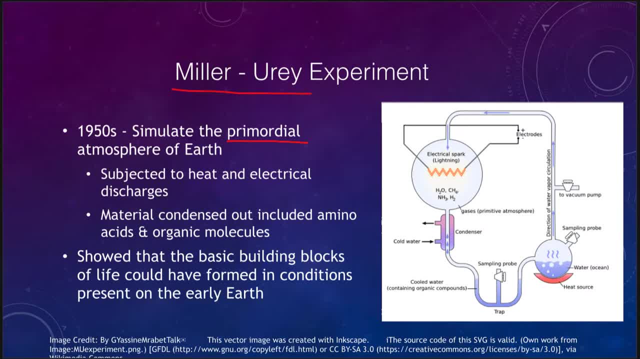 what would have been present, things like methane and ammonia and water and hydrogen that would have been present in the simulated, in the sorry, in the early atmosphere of the Earth. So we simulate that here We put the atmosphere, those gases that we believe would have been. 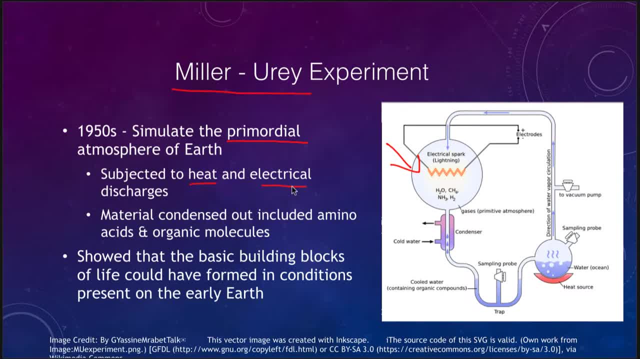 present. We subject them to heat and electrical discharges, as would have occurred in the early Earth, that we would have had, You know, we would have had, you know, we would have had lightning storms, we would have had more heat. And what we do is then run the water, run water vapor through it. So the water vapor runs through And as it condenses out, there's a trap here where we can contain anything that forms. So what we see in this trap is that we find amino acids and organic molecules that form from these basic compounds that we know would have been present in the 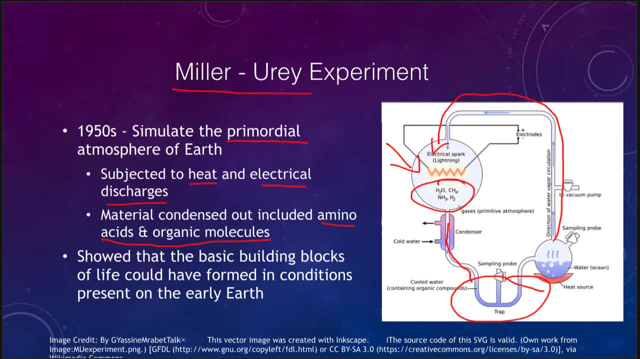 early Earth's atmosphere. So what we see is not necessarily that life is easy to form, but that the basic, basic building blocks of life can't could have formed on the conditions present in the early Earth, And these compounds are not unique to Earth, so they likely could have formed elsewhere. So we see that the building blocks of life are very common. What we don't know is how common it is for life itself to actually form. 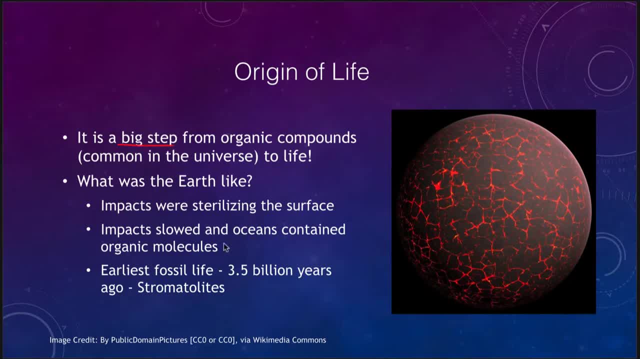 So how do we do that jump? It's a very big step from organic compounds which are very common to life. Life is something that we don't know of other than here on the Earth. So what we want to look at is: what was the early Earth like? At the time, the Earth might have looked something like this very hot molten impact constantly being impacted And that was sterilizing the surface, So life was unable to form very early on. 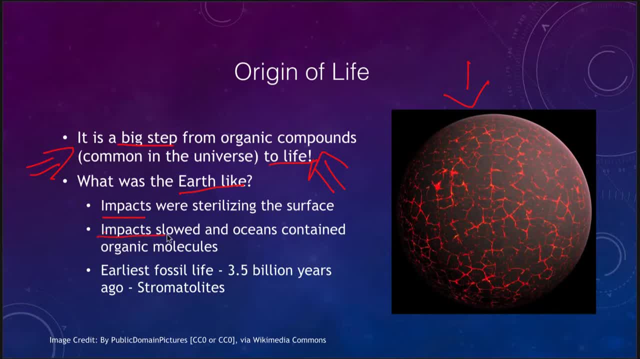 However, over time, over that first few 100 million years, the impact slowed and the oceans began to form, And in the oceans we would find organic molecules, much as we saw with the with the Miller Youri experiment. So what we see- one of the things that we find- is that early fossilized life actually occurred very early on in the history of the Earth. We believe life actually took place on trusting gebrucus, Here's the proof of ducks, and we're going to go through this to make sure if it's right or not. So let's go and see. As I said, 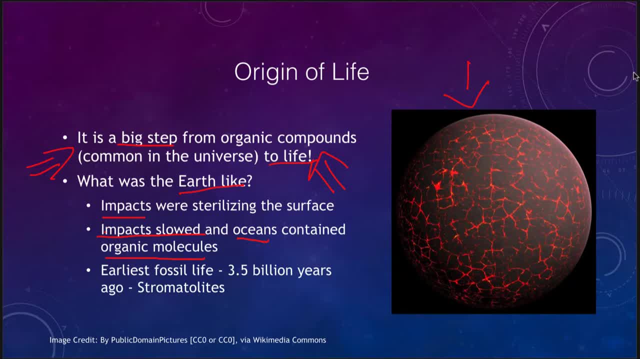 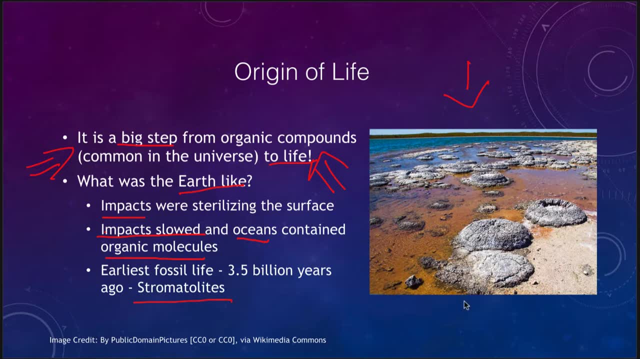 life itself may have formed earlier, but we have to see what was actually able to form, And one of the things that we see are these stromatolites And these objects here are actually formed very early on, and fossilized remnants of them have been found dating back. 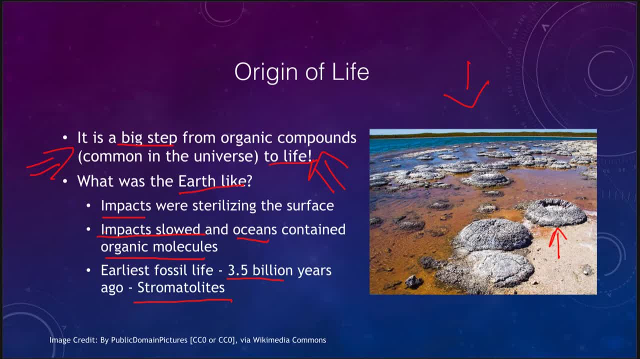 to three and a half billion years. These are some of the very oldest objects that we see, various oldest evidence of living objects. Now likely life had to exist before these, so life formed. if the earth is four and a half billion years old, it had to have formed. 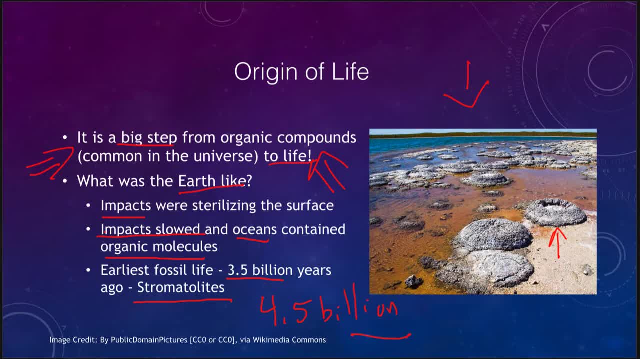 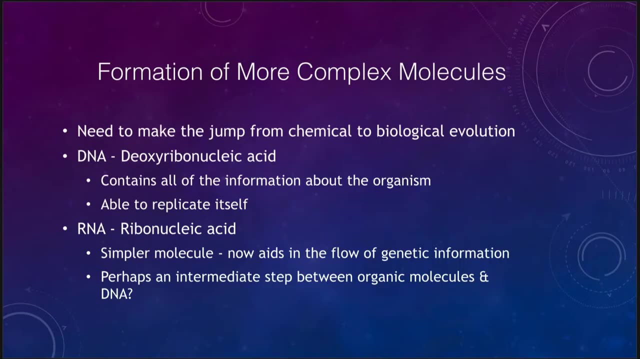 very shortly after the earth formed itself. So it seems like there has been life on Earth for the vast majority of the time that the earth has been around. So we see some of this early evidence from long ago. How do we form more complex molecules? 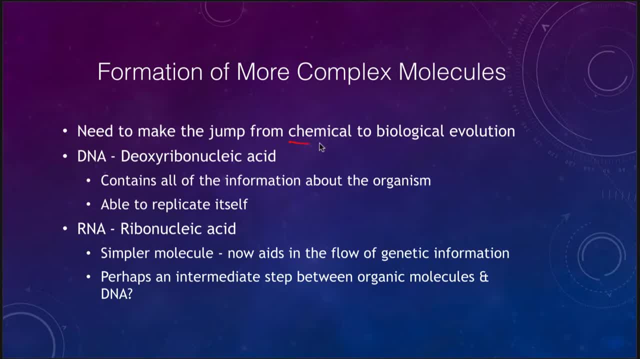 We need to make a jump. We need to jump from chemical evolution- which is what we've been looking at in things like the Miller-Urey experiment- to biological evolution. So there's a big jump there. you can have chemical reactions that can make these compounds, But how do? 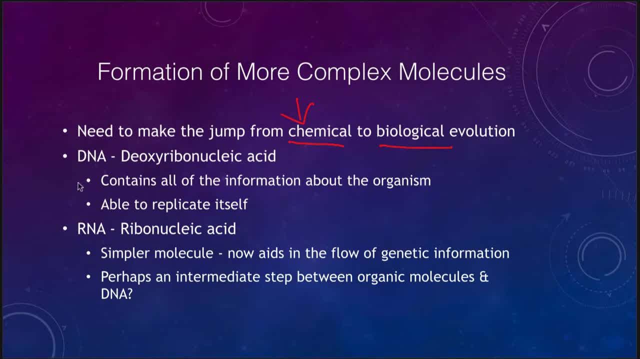 we get that into something that is actually living. One of the things is the DNA, which contains all of the information about the organisms. It's built on the amino acids that we've already talked about, So you put the amino acids together in the right pattern. 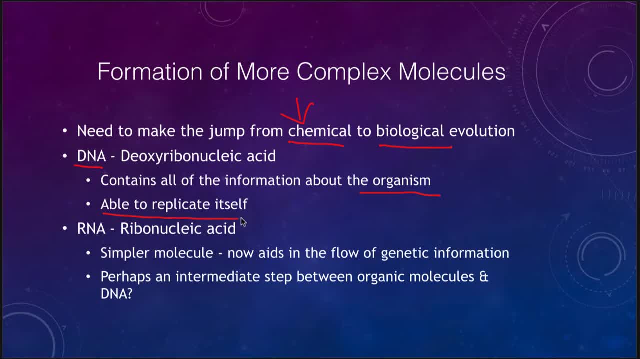 And this molecule is able to replicate itself. One of the beginning signs of life is that there it is able to reproduce. So when we talk about chemical evolution, we don't have any reproduction going on. Here we actually have reproduction. the DNA can split itself. 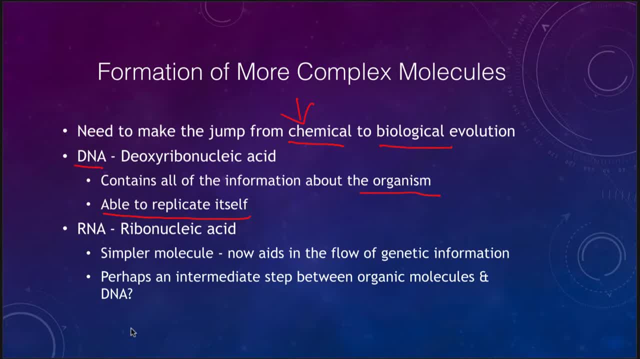 and replicate itself and make identical copies. You also have the RNA, which is the DNA, that is a simpler molecule which aids in the flow of the genetic information. Could this be some kind of intermediate step between the organic molecules? Again, we said that these 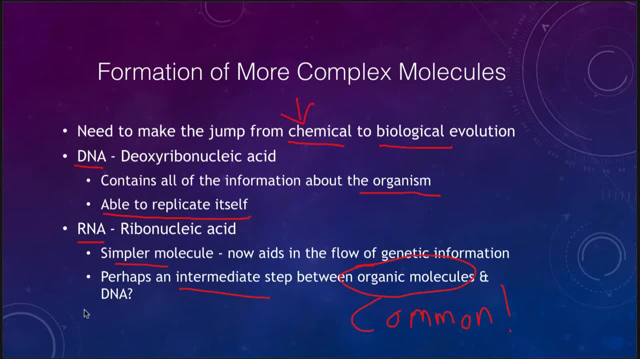 are common to DNA and then to life. So how do we get it? Could this be an intermediate step leading to life? Now, one of the things that we see on Earth and that we associate with life is oxygen. What do we see about oxygen in the atmosphere, And what we find is that, for the vast majority, 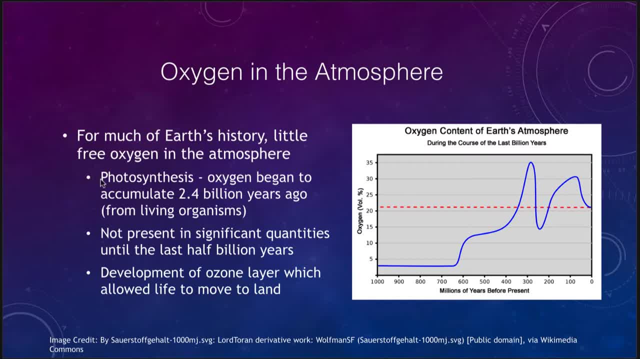 of the Earth's history, there was very little oxygen in the atmosphere. Oxygen was tied up, maybe, in things like carbon dioxide or water, But if we look at the percentage here, very, very small. until about 650 or so million years before the present, that's only the. 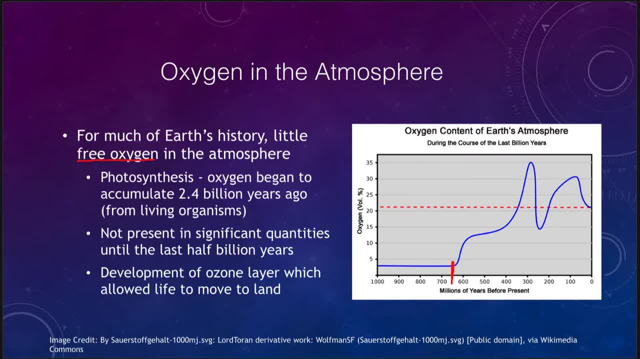 last half billion years of the Earth's history, So at the time of the very earliest life, there was no oxygen in the Earth's atmosphere. Now it took time and the oxygen content has then come up and then settled down to about the 21% we know of it today. But this is about the time that photosynthesis began early on. 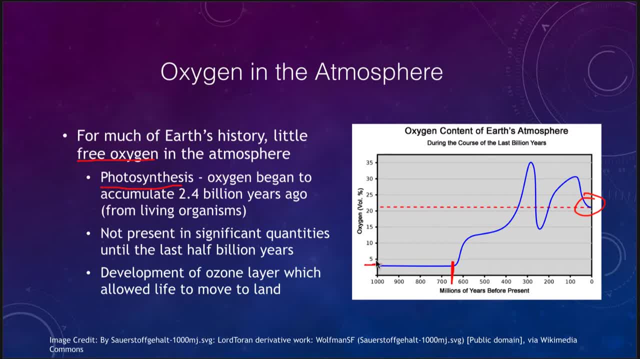 and oxygen began to accumulate. So we had a very low level of oxygen even 2.4 billion years ago, but it would not have been sufficient for us to be able to breathe. It's only at about a 3% range of the Earth's atmosphere, So would not have been sufficient. 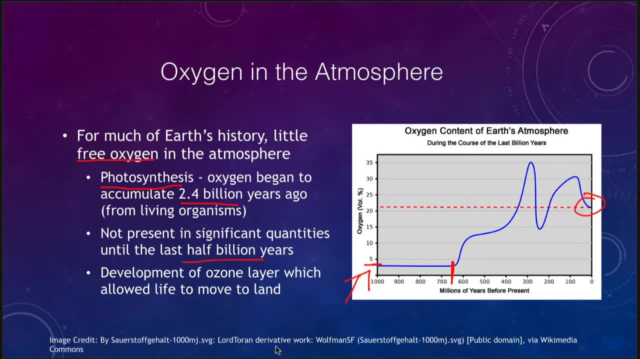 oxygen for us to breathe, And it hasn't been until the last half billion years that we've actually gotten significant quantities of this. The development of free oxygen- meaning not tied up in other molecules- meant that we actually formed the ozone layer, which 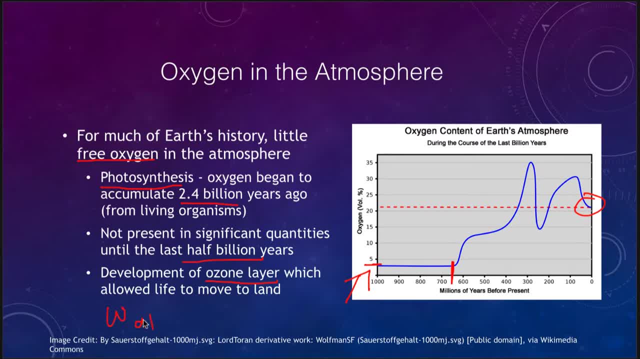 allowed life to move from water, where life had existed for most of that, to land, And that was the development of the ozone layer, which protected us from ultraviolet radiation. Ultraviolet radiation very damaging and sterilizing and would rip apart these 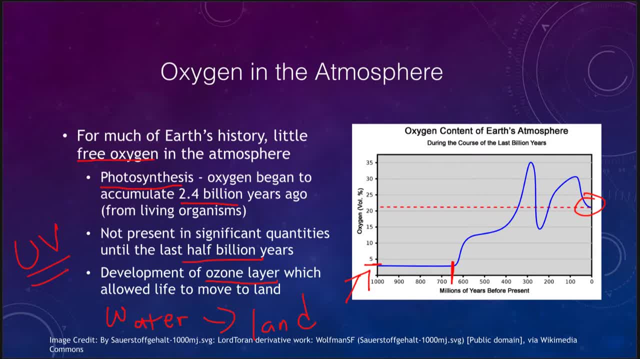 organic molecules as they formed, especially out on land, without the water in the ocean to protect them. But the development of the ozone layer, absorbing a lot of that ultraviolet light, then allowed life to move on to land, And that's what we begin to see here shortly. 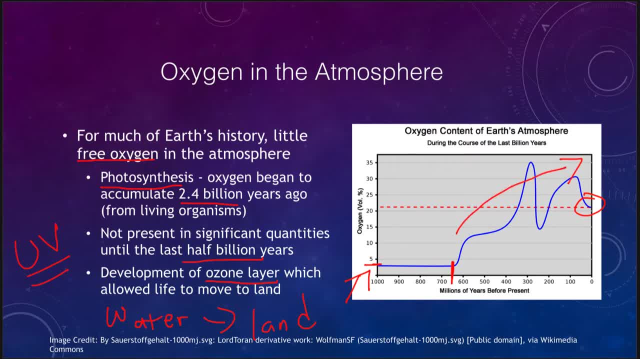 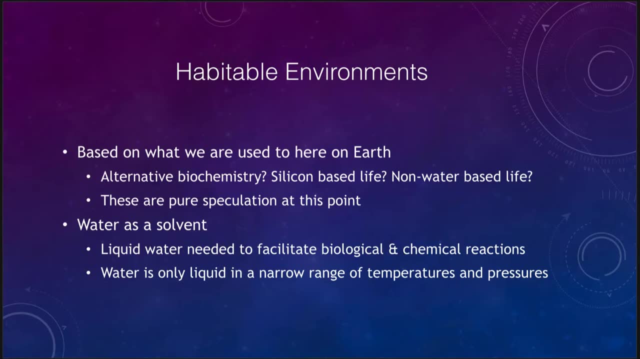 after life begins to move from the oceans on to land. So, while life existed on Earth, for the vast majority of Earth's history life was only in the oceans. Now, when we talk about habitable environments, what do we mean? They're based on what we're used. 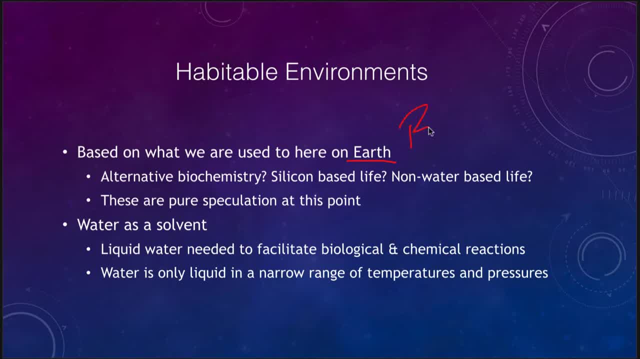 to here on Earth. So we are opening our own form of bias. We think, perhaps, that life in the universe has to be something like us Possibilities of alternative biochemistries. Science fiction is good about putting things like silicon-based life, life based on silicon instead of carbon, because silicon shares. 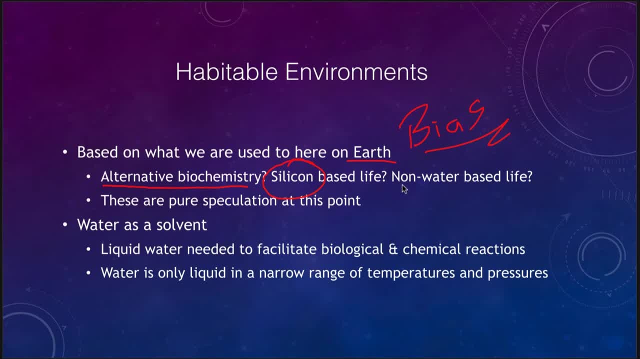 some chemical similarities to carbon? Can you have life that is based on some other liquid that is not water? But these are really all speculation. We have no idea until we can actually someday maybe get out there in the universe to see what is going on. 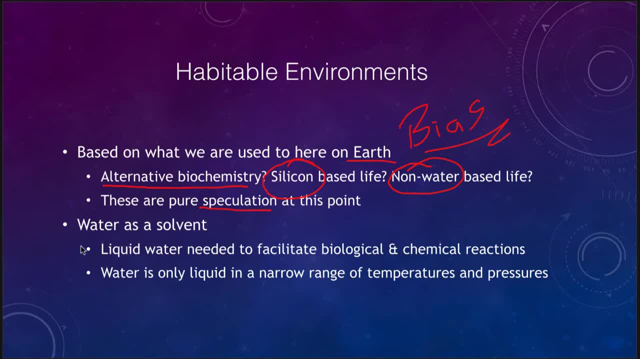 What other types of life there might be. We like water as a solvent because it is needed. Some kind of liquid is really needed to facilitate biological and chemical reactions. If you dry out the organic molecules, they're not going to react together and form great chains. 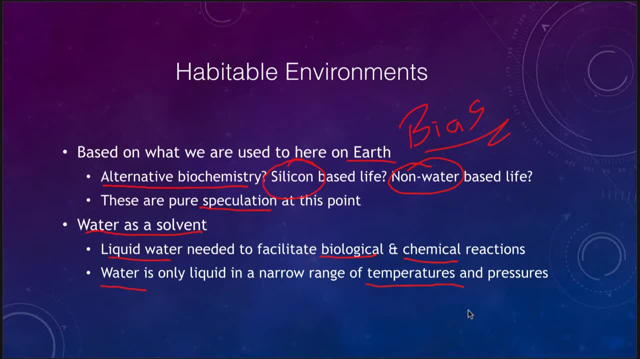 Water happens to be liquid at a very narrow range of temperatures and pressures, So it's not necessarily common as a liquid. Liquid is very common in the solar system, either as a gas or a solid, but liquid exists only that we know of here on the Earth. So other liquids, things like methane, exist. 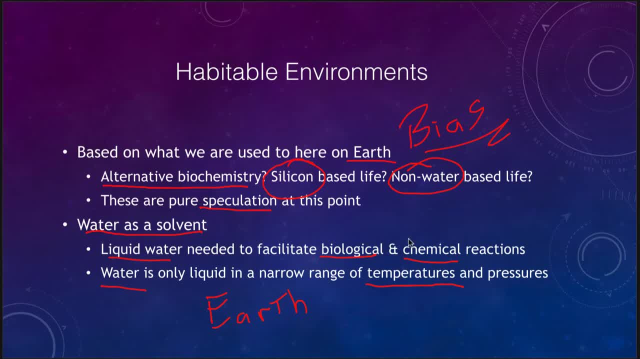 on Titan, but the temperatures are much colder, And when temperatures are colder, reactions seem to go much slower. So the reactions would go slower. Would it be as likely for life to have formed someplace where the temperatures are bitterly cold, even if you did have a? 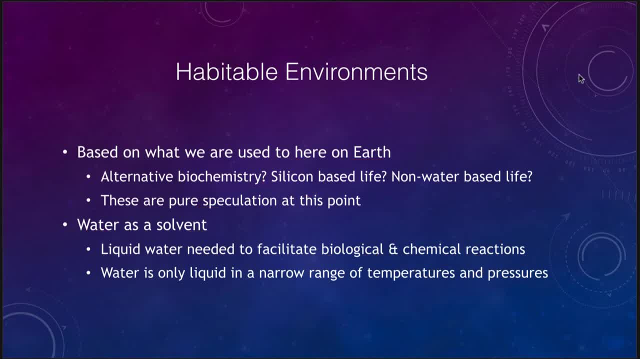 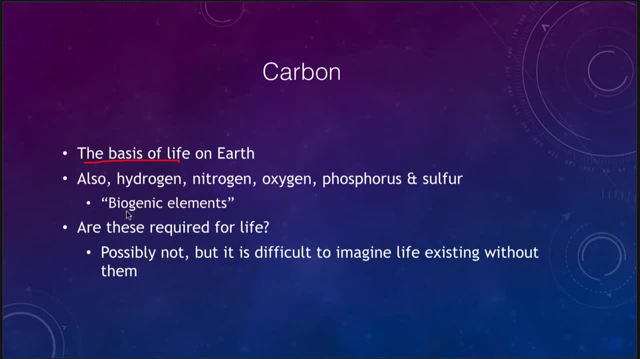 liquid. So water is one thing we look at, Another is carbon, And carbon, again, is the basis of life on Earth. We also use what we call the biogenic elements, which include hydrogen, nitrogen, oxygen, phosphorus and sulfur, which are very primary elements needed for. 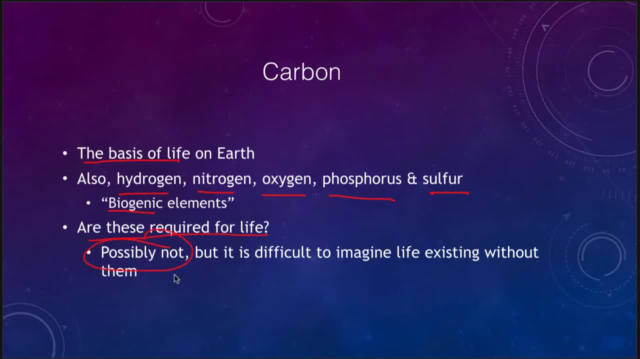 life. Are they required? Maybe not. Maybe we can imagine life built on something else, But it's hard to figure out exactly how they're built. But it's hard to figure out exactly how they're built. But it's hard to figure out exactly how they're built. 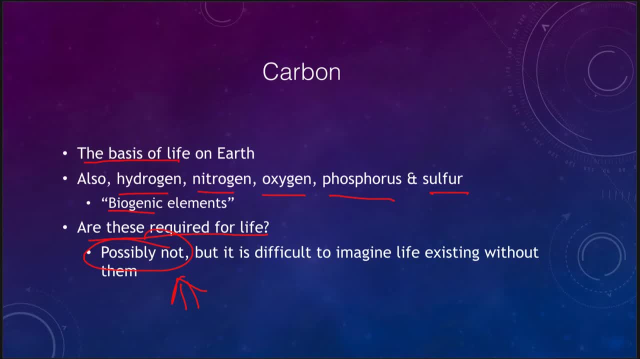 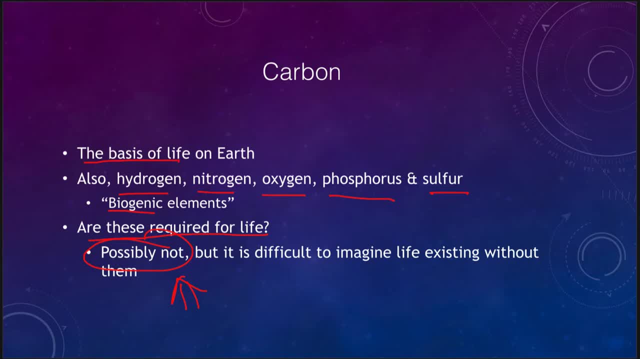 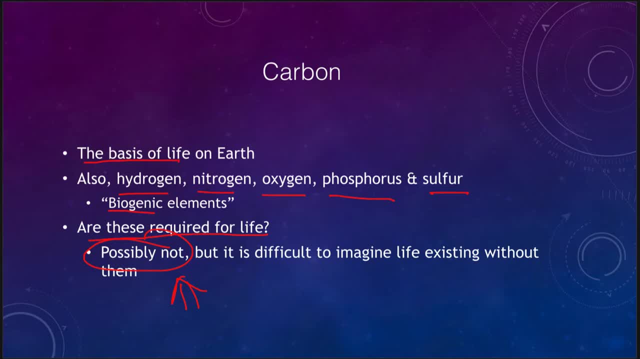 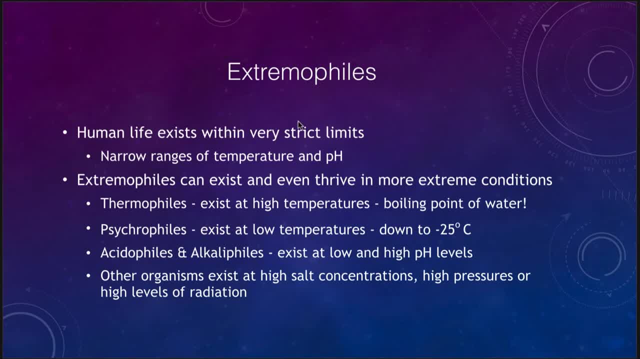 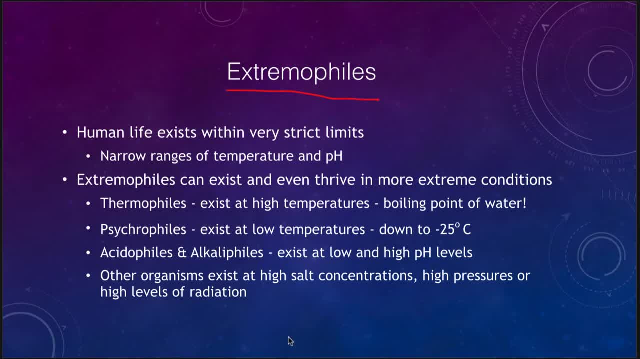 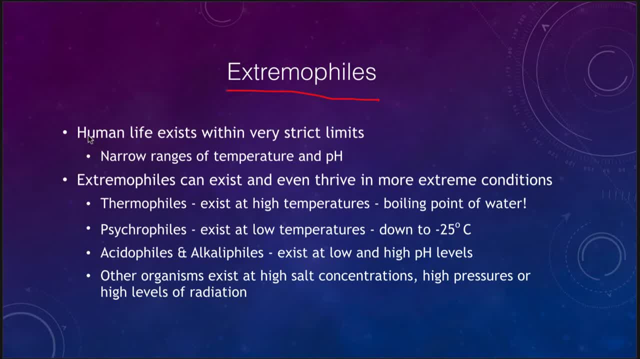 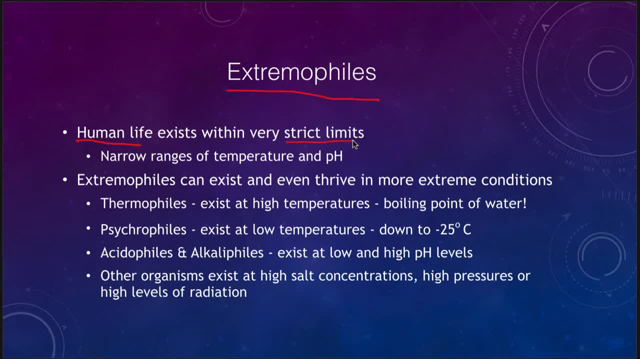 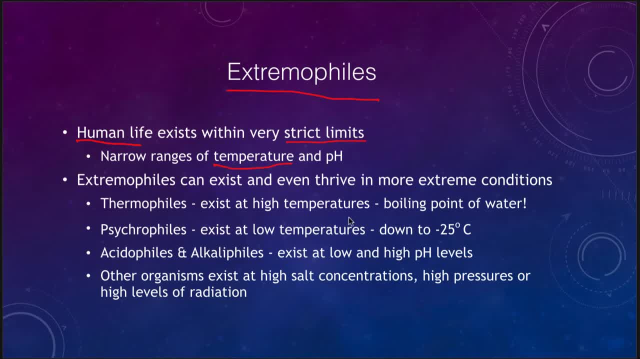 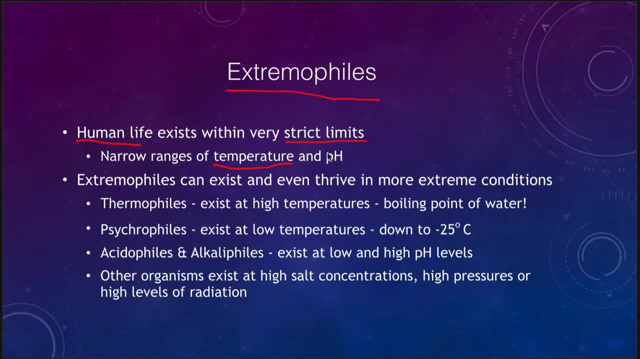 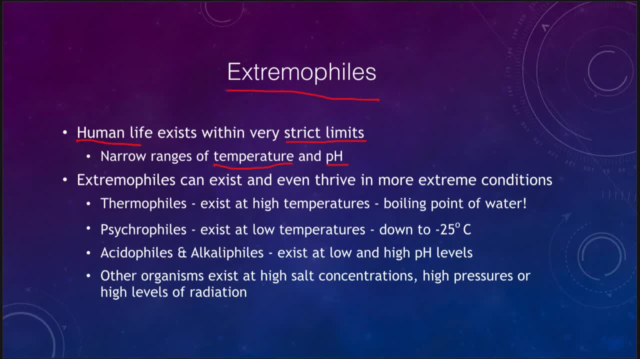 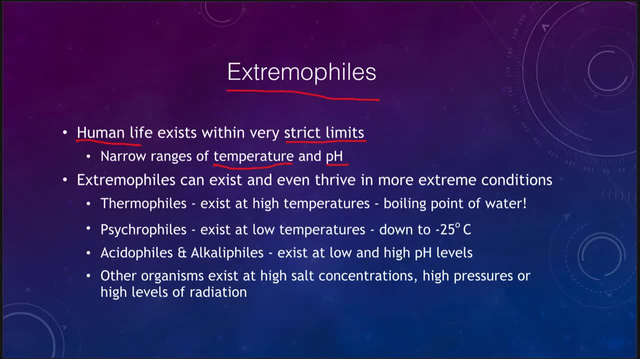 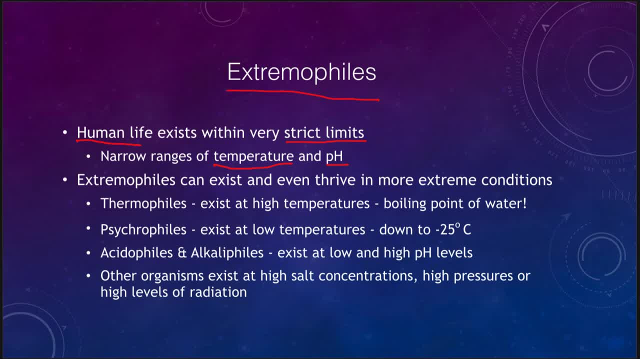 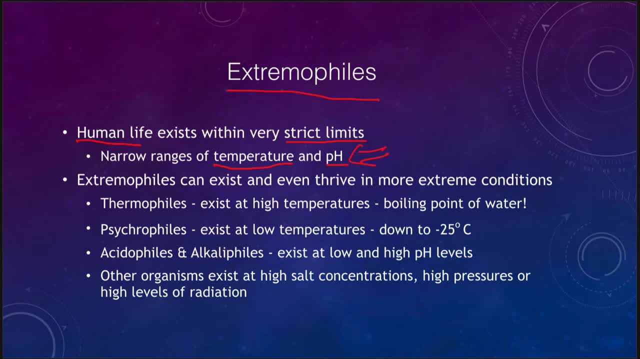 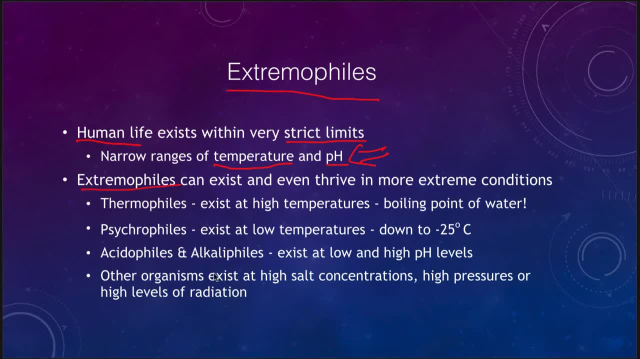 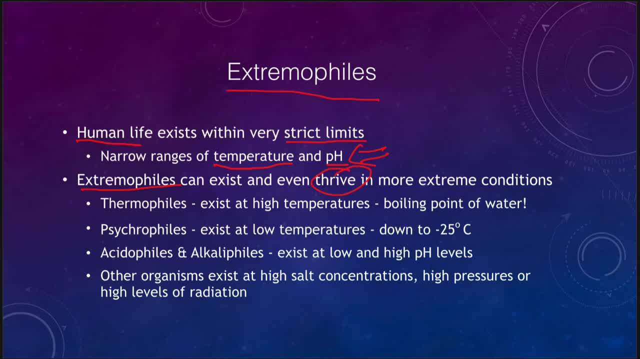 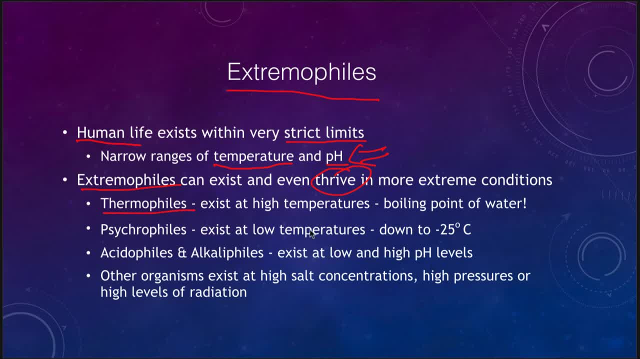 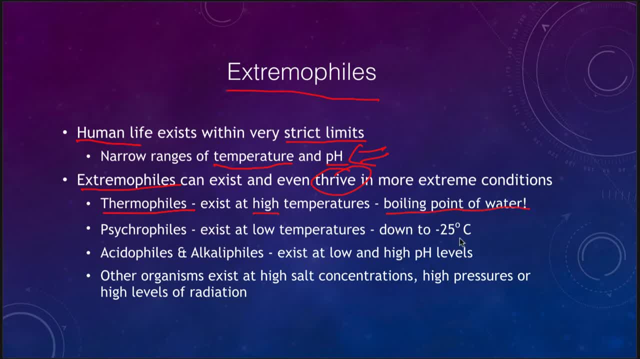 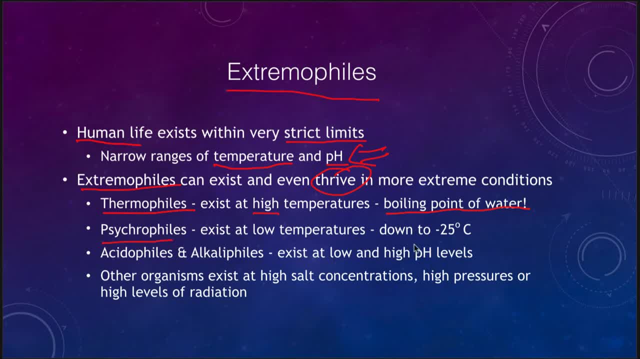 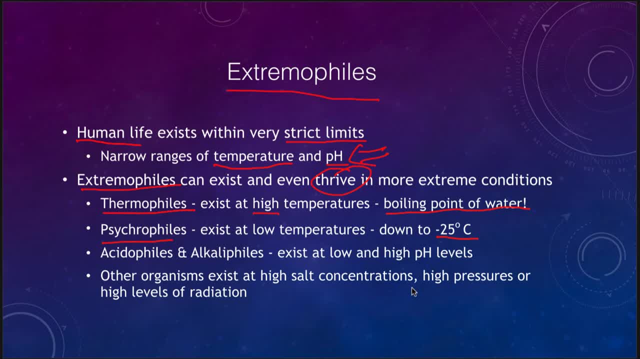 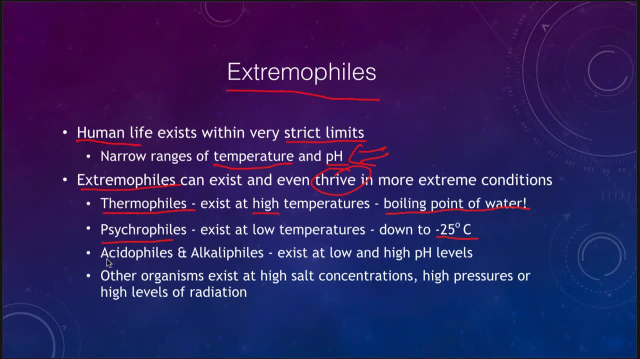 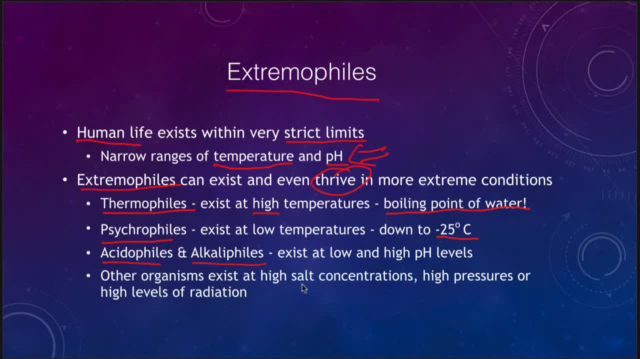 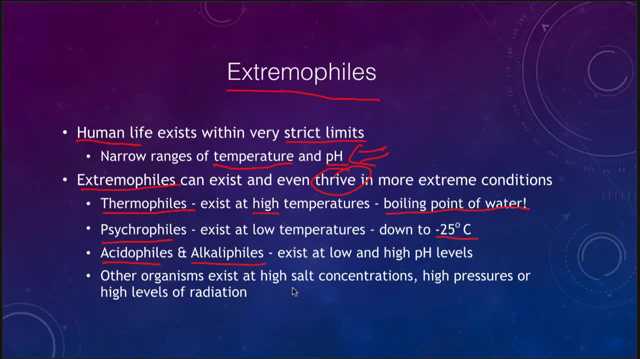 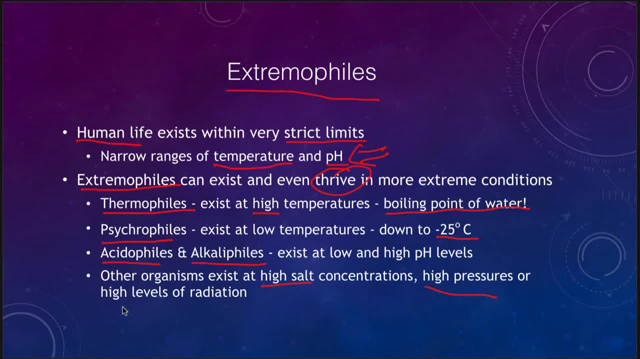 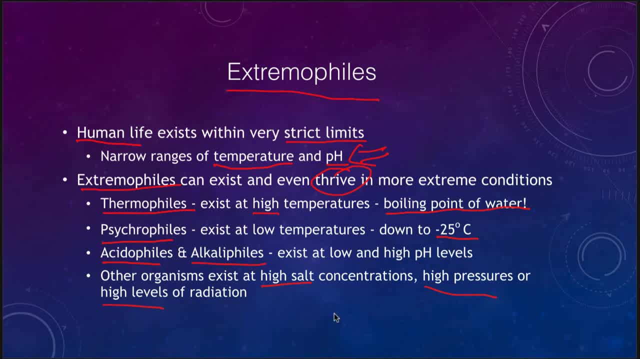 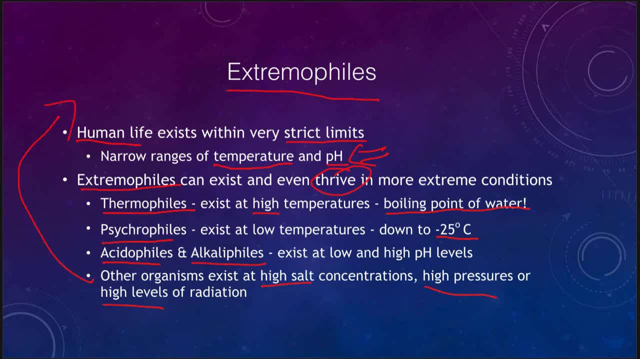 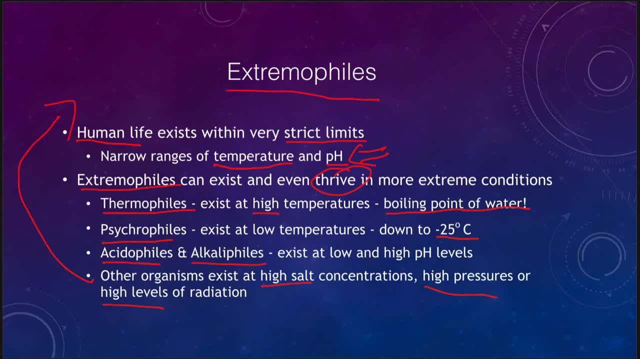 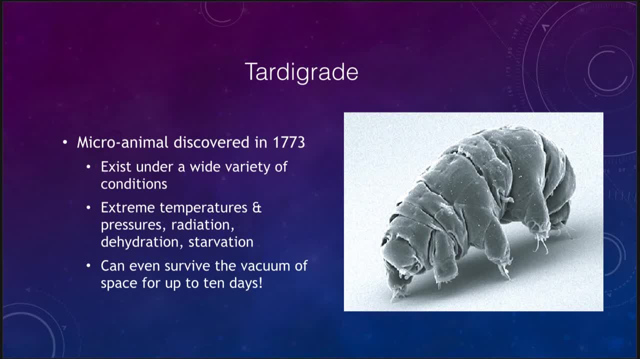 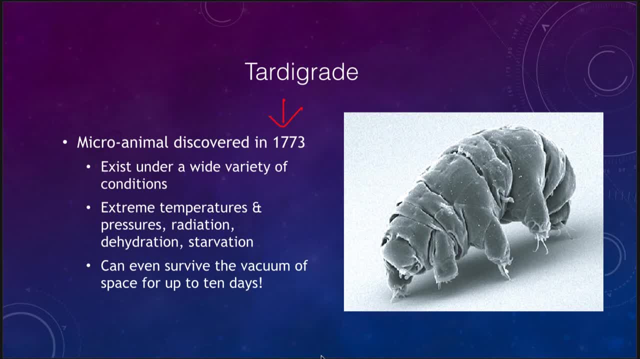 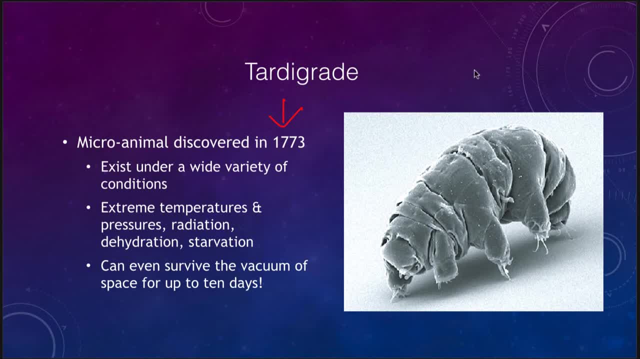 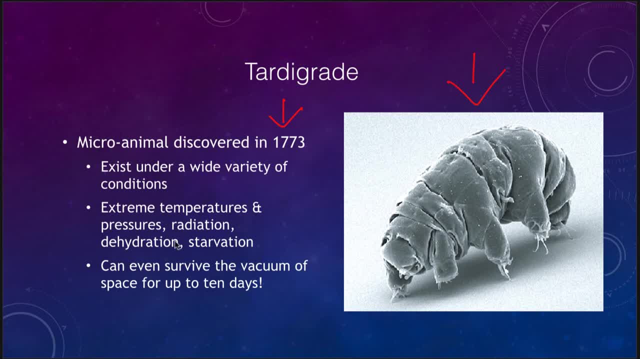 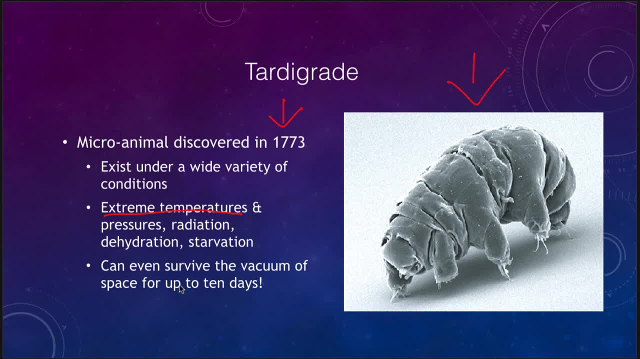 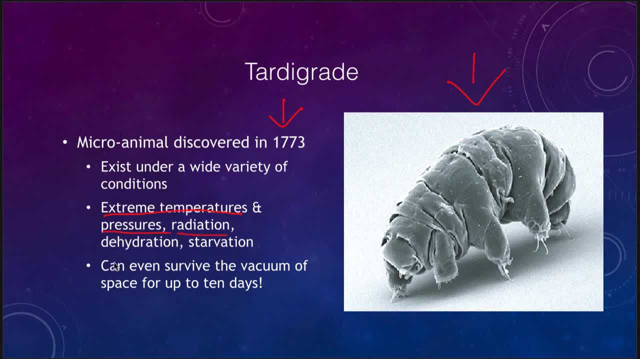 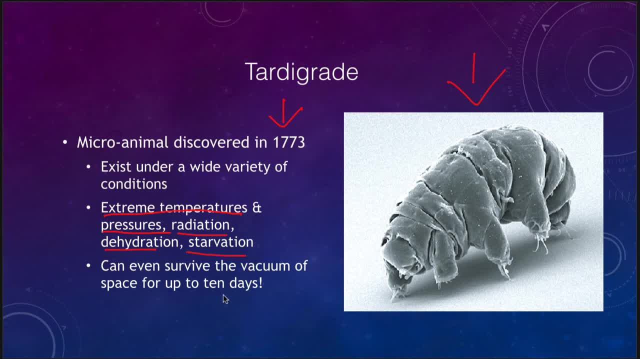 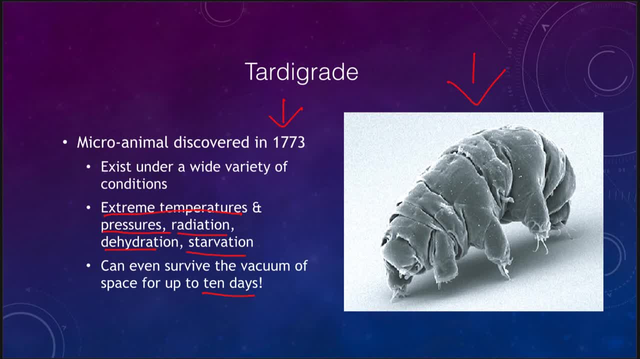 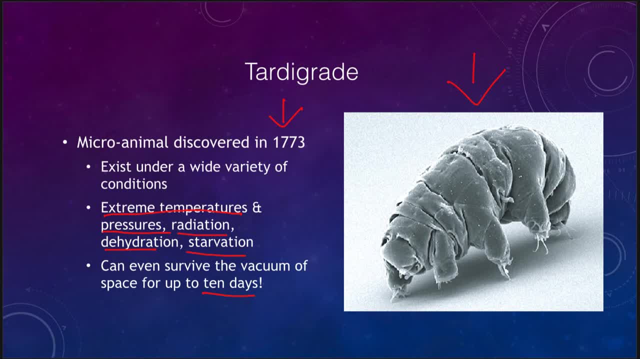 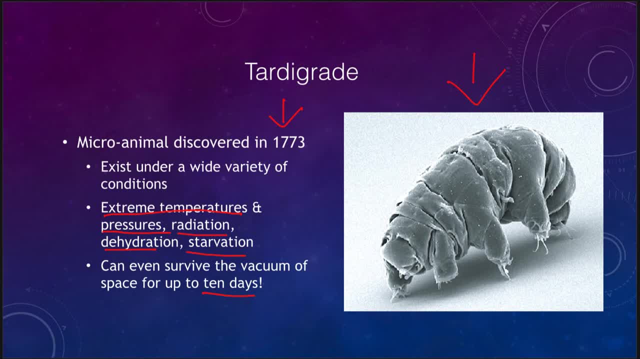 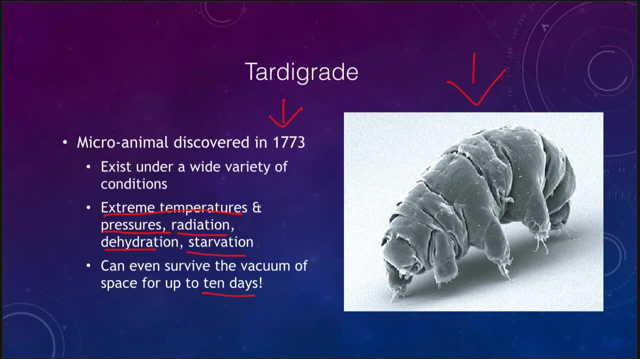 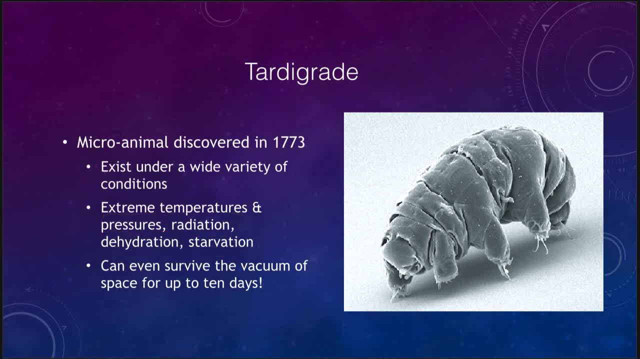 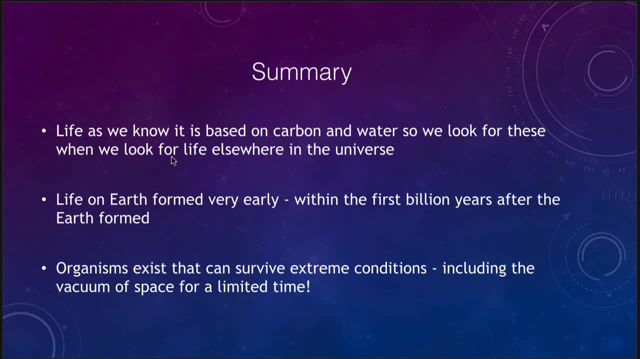 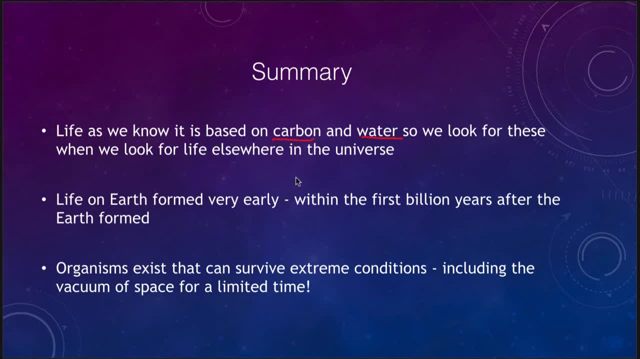 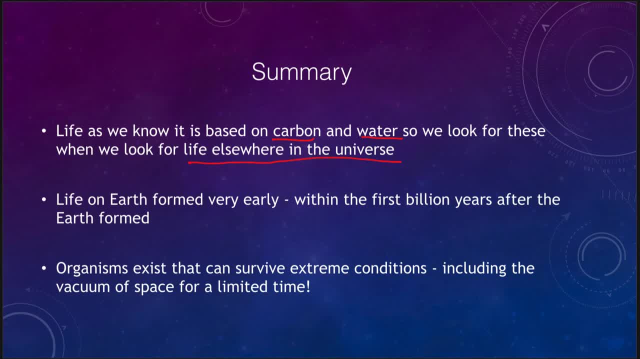 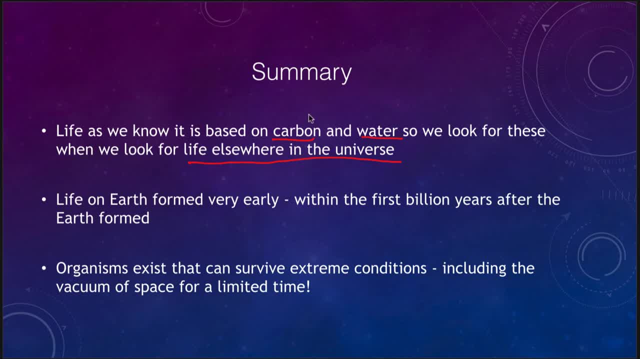 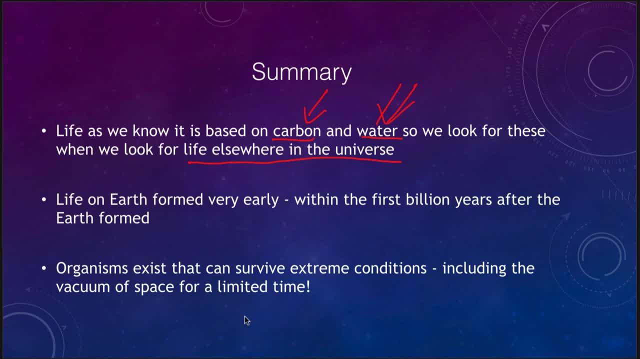 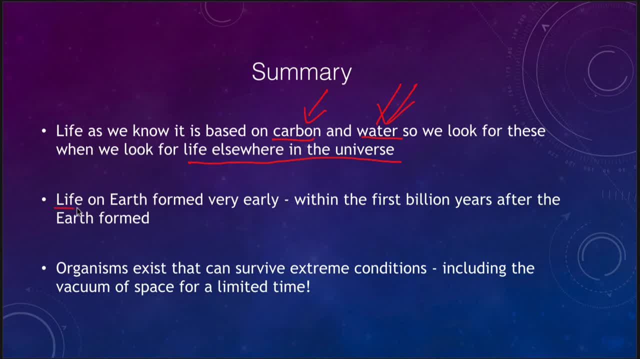 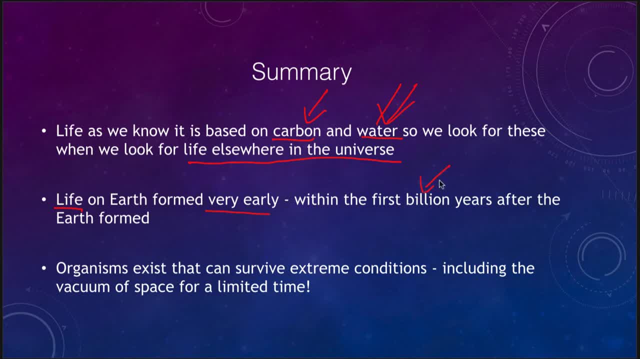 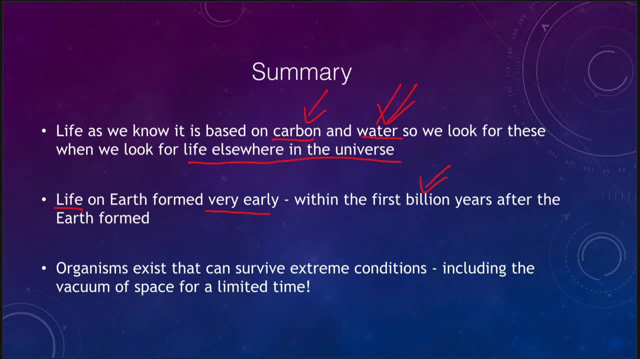 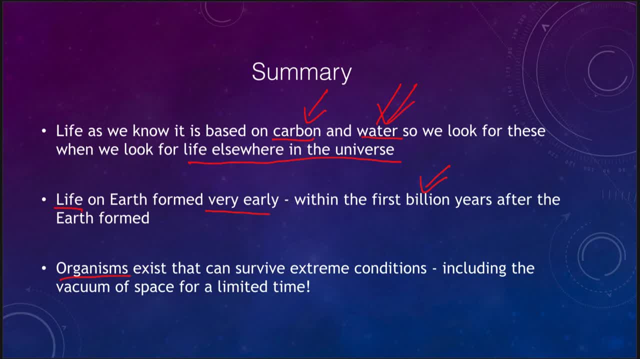 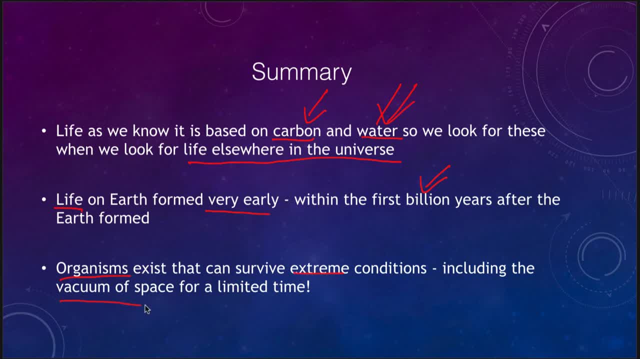 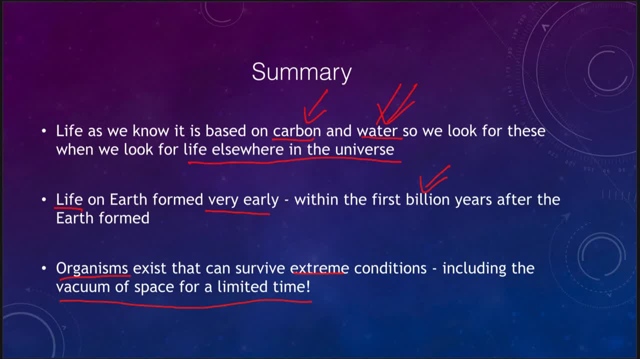 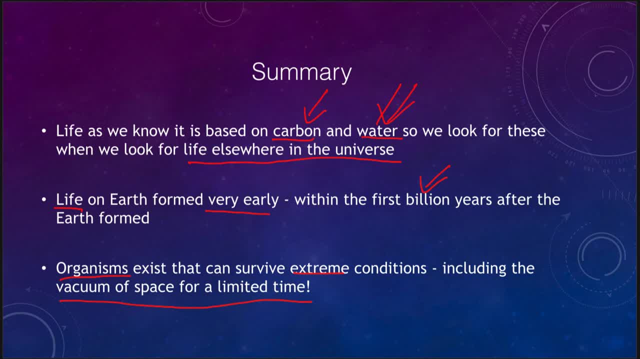 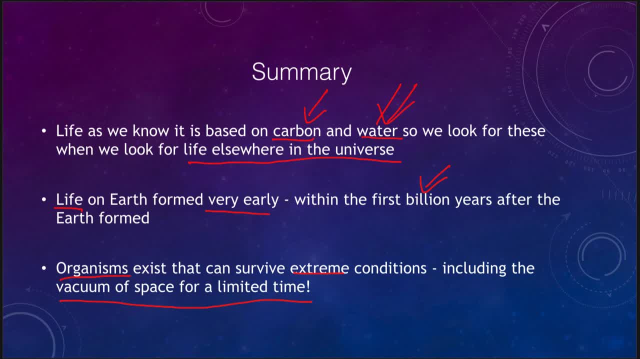